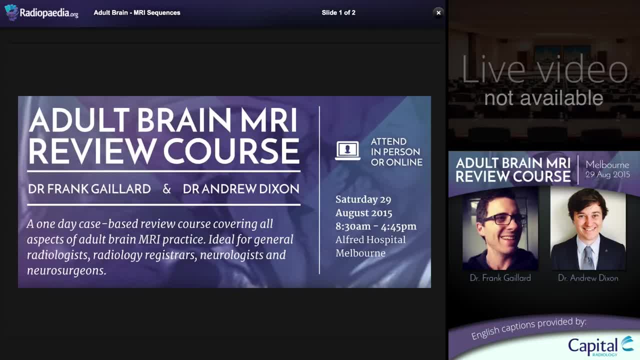 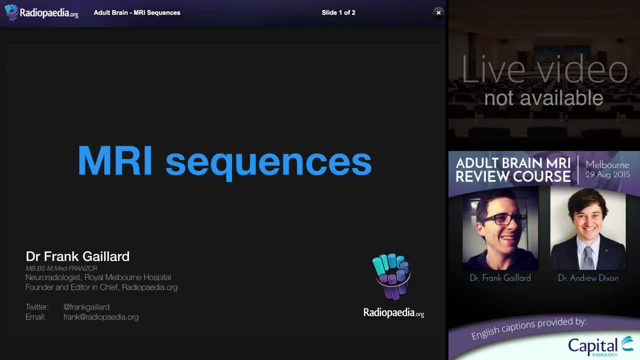 the actual live presentation and during the remainder of the videos, A degree of familiarity with MRI sequences is expected, and so this talk is really just to make sure that we're all on the same page. I'm not going to be going into a great deal of detail into any of the sequences, and in fact we won't be. 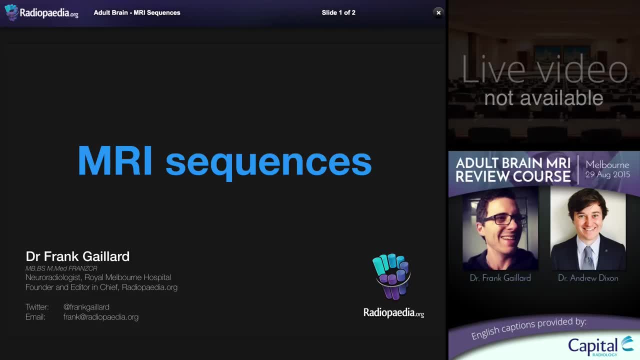 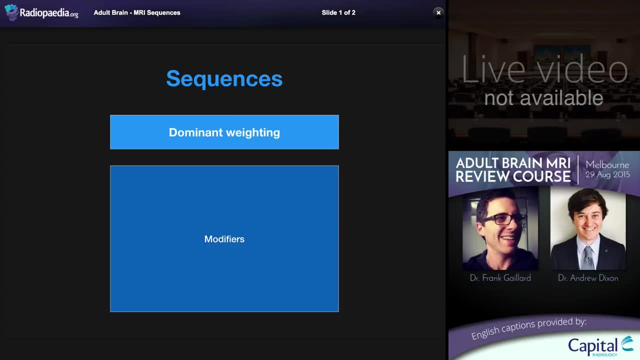 touching on any of the physics, but just to ensure that we understand the appearance of all of the main ones and the terminology used. There are a great number of MRI sequences, so much so that I think, in many ways it's easier to consider MRI a collection of modalities, because the 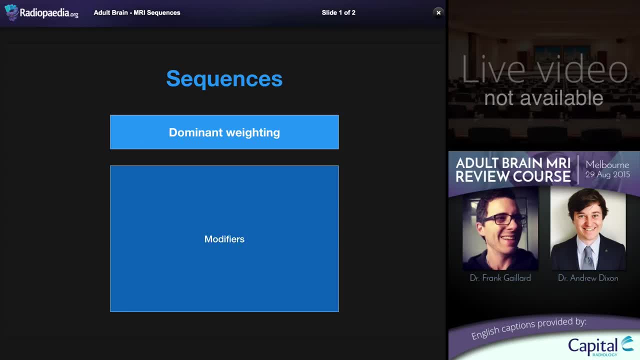 differences between MRI and MRI are so many that it's very difficult to understand. the differences between different sequences is almost as large, if not larger, than between some different modalities. So when we talk about sequences, there's no single way of grouping them or of discussing them. but 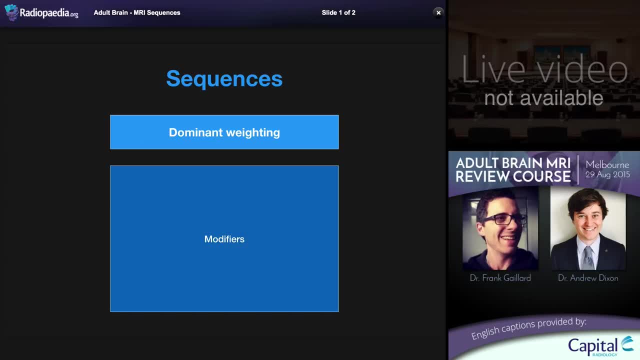 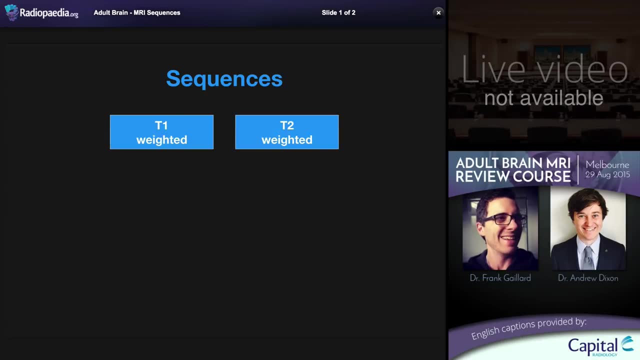 a useful one is to think about what the dominant weighting or the dominant characteristic that's been examined, and then there's a number of modifiers applied to each of these, So let's start with the main two that we are used to thinking about: T1 weighted and T2 weighted. These are the two fundamental. 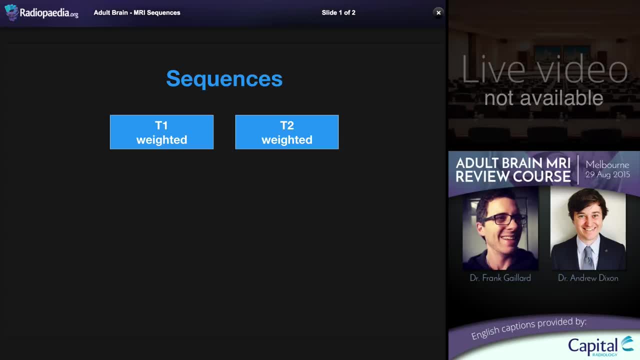 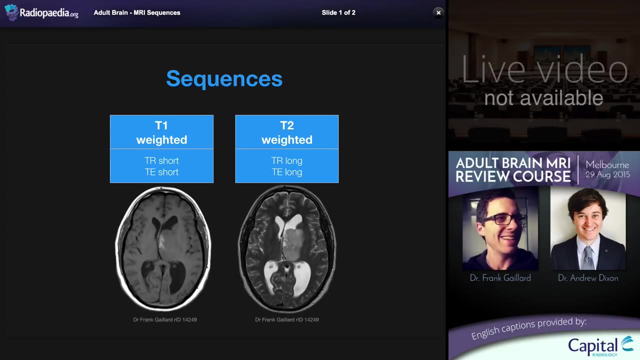 anatomical sequences upon which many other sequences are built, and different tissues have different appearances depending on which sequence is chosen. They are characterized by specific TR and TE intervals, with T1 being short and short and T2 being long and long, and this is their typical appearance. The 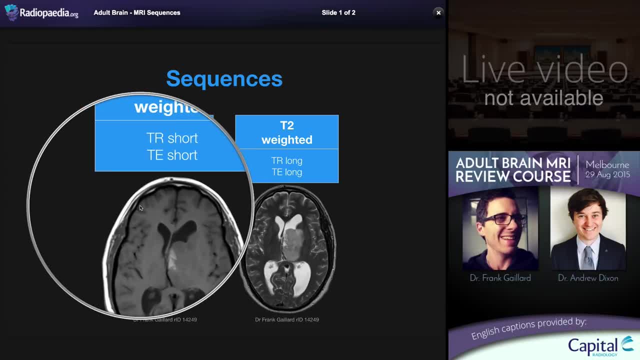 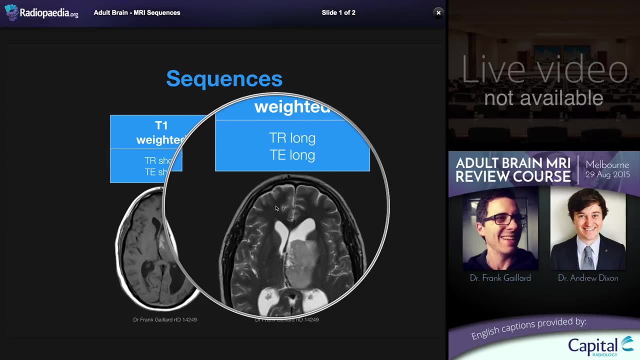 easiest way to identify a T1 weighted sequence is to examine the relationship between white matter and gray matter. Where the white matter is whiter, then the gray matter. So they match: the white matter is white and the gray matter is gray. In contrast, T2 weighted sequences have the opposite. 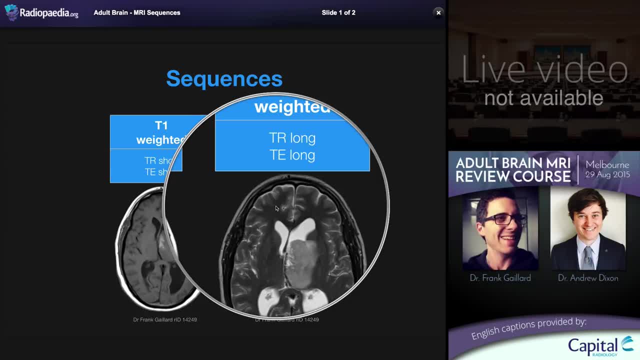 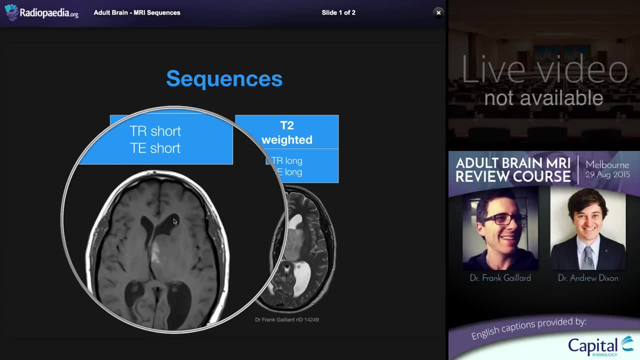 relationship with the gray matter being more hyper intense compared to the white matter, which is really quite dark. And yes, of course the CSF is bright on T2 and dark on T1 but, as we'll see shortly, that's not always the safest way of. 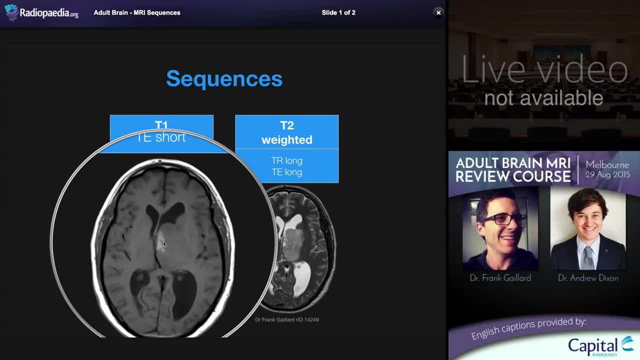 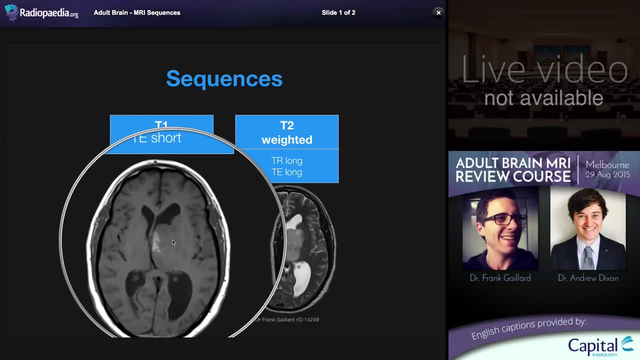 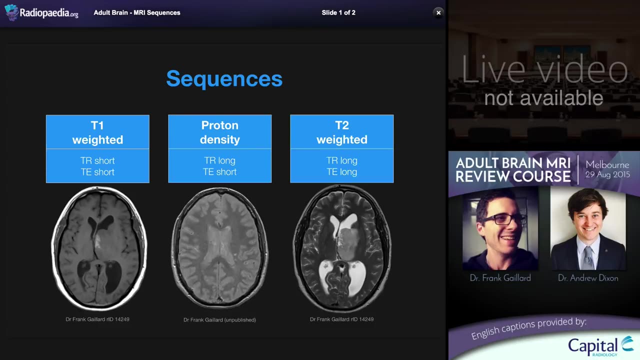 identifying them. A number of substances are hyper intense on T1 and T2.. With the ones most relevant to the brain being blood product, fat, some proteinaceous material and contrast enhancement. Proton density is an intermediate sequence characterized by a long TR but a short TE, and has 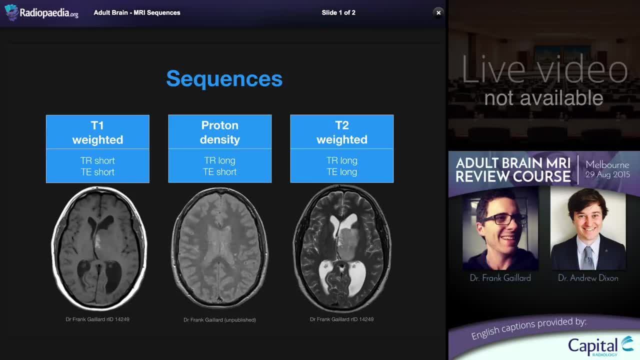 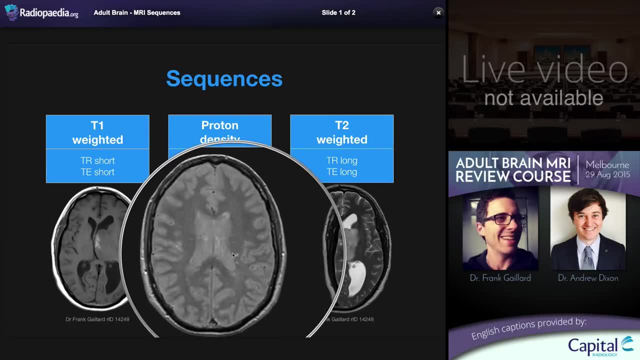 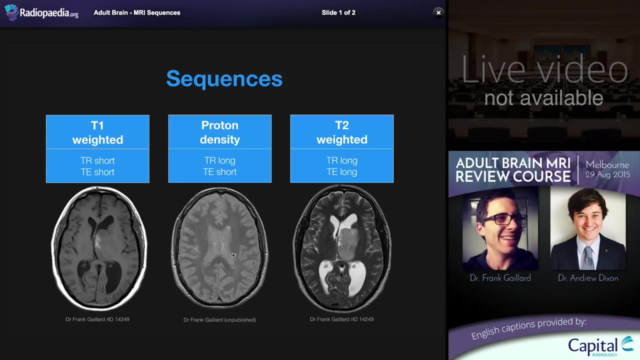 appearances that were very useful in the early era of MRI in examining white matter, Making white matter lesions easier to identify than T2 or T1.. The role of proton density has largely been superseded by flare imaging or fluid attenuated inversion recovery to the point that very rarely is a proton. 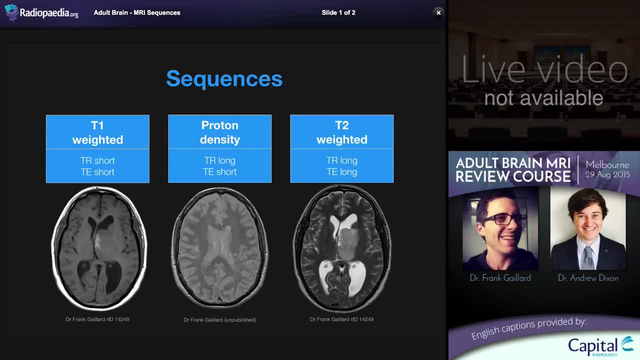 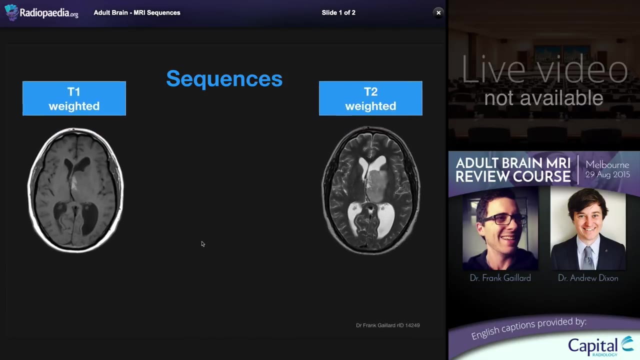 density performed in modern-day protocols, So essentially, we can forget about proton density brain imaging as of being only of historical value. It's important to note, however, that proton density as a sequence is still alive and well in other parts of the body and is particularly useful in musculoskeletal. 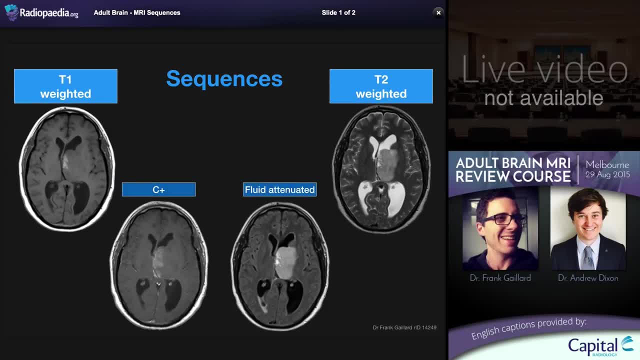 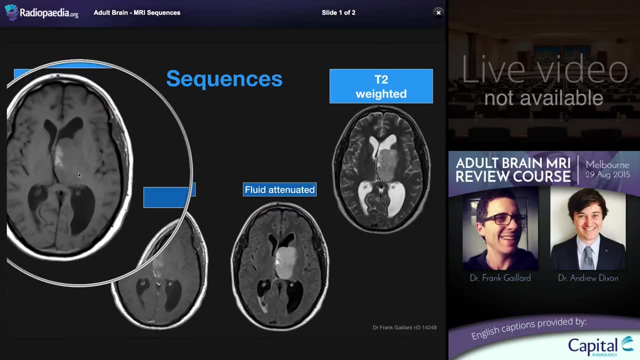 So if we take T1 and T2 weighted imaging, we can see the first ways that we can modify these images. The first is to add gadolinium and then perform T1 weighted sequences, In this case where we have a thalamic primary brain tumor with some 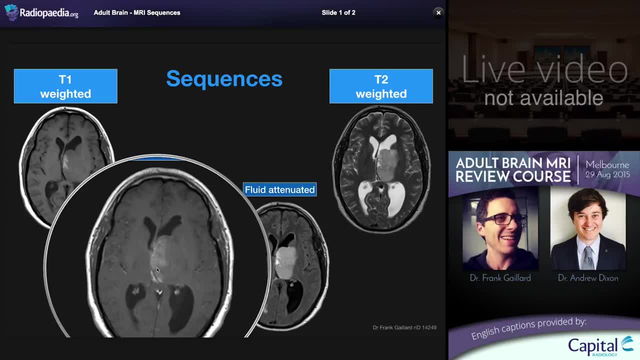 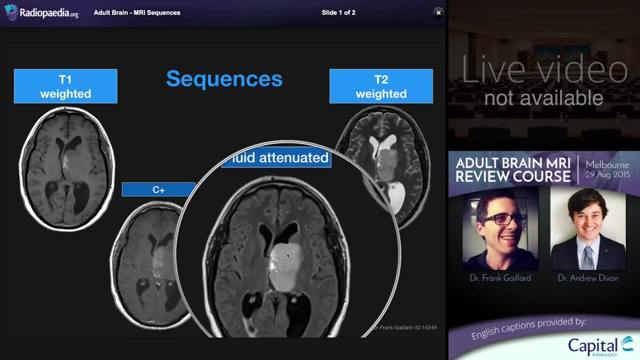 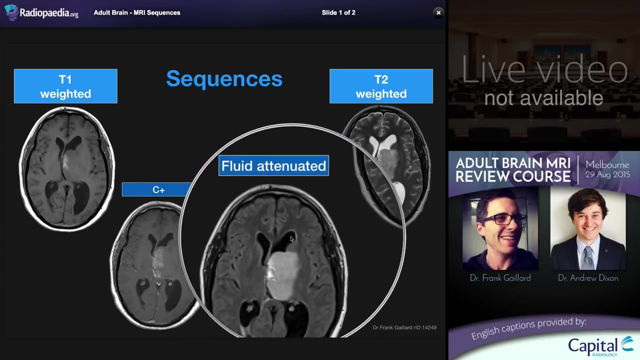 hemorrhagic change which has intrinsic high T1 signal, we can see that another component of it demonstrates contrast enhancement. The most common modifier for T2 weighted images is fluid attenuation, Usually referred to as flare for fluid attenuated inversion recovery. And here we see this same tumor standing out more brightly against the white matter and 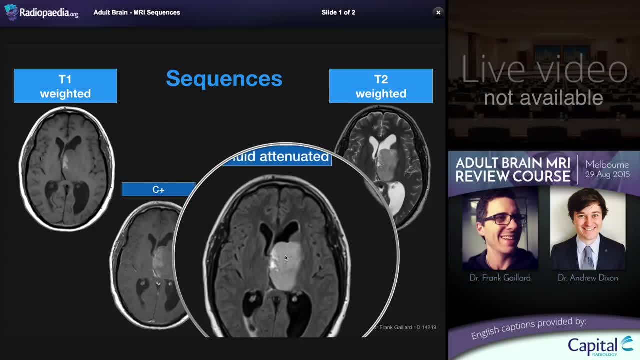 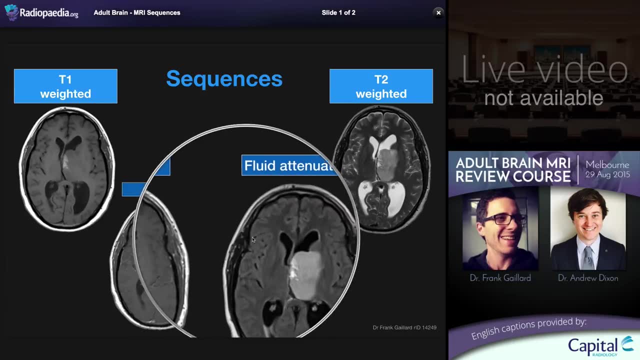 adjacent brain parenchyma, now that the CSF within the ventricles has been attenuated. Note that despite the attenuation of a CSF, such that it is dark, similar to the appearance on T1,, the relationship of the white matter to the 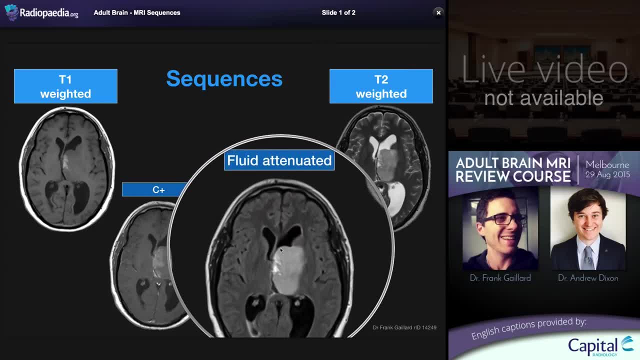 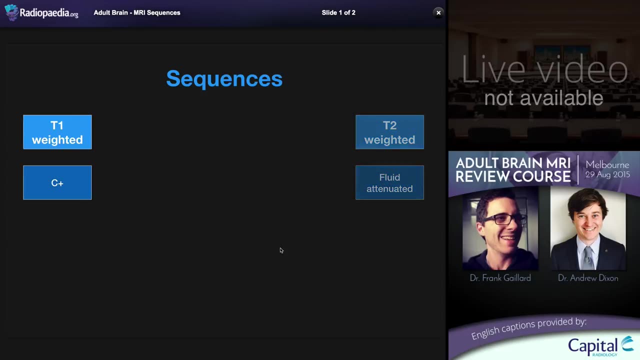 gray matter has remained that of a T2. weighted sequence, And this is why this relationship is more important and an easier way to identify T1 versus a T2 weighted sequence. Otherwise, a flare sequence can be mistaken for a T1.. The next, most important way that T1 images. 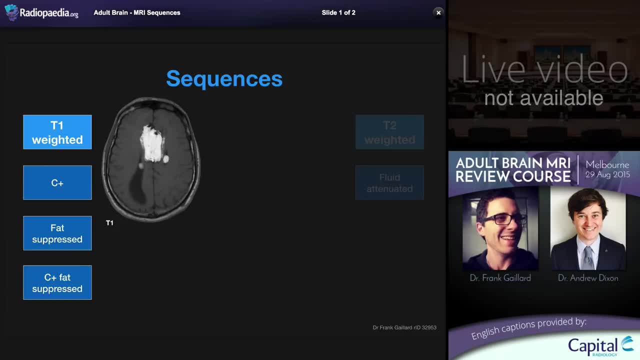 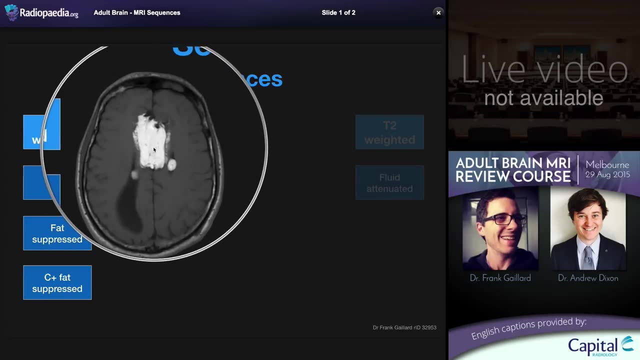 can be manipulated is to apply fat suppression, And this can be done both on pre-contrast or on post-contrast images. Here we have a case of a pericallosal lipoma with a large amount of very hyper intense fat seen in the midline. 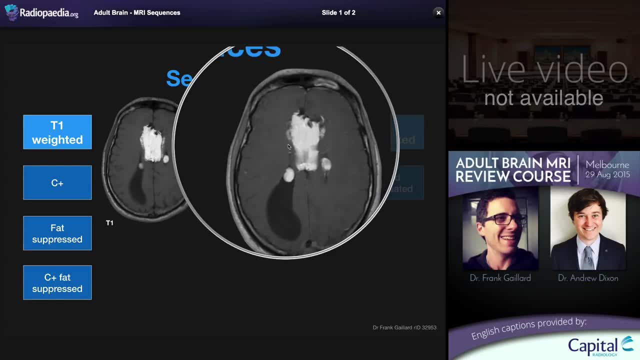 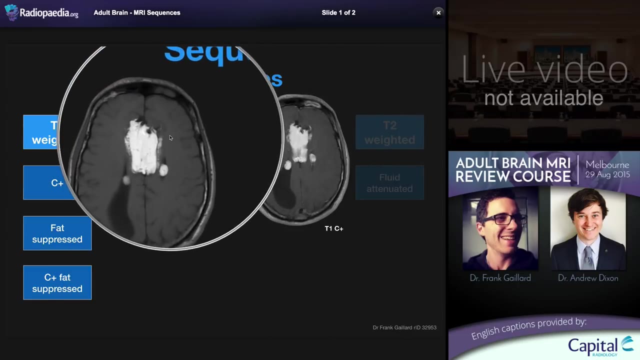 When we perform contrast, it is a little bit difficult to tell whether there is contrast enhancement at the margins or whether this represents merely fat. The slice position is not always the same, so an exact comparison is difficult. One could assume that this is enhancement, but one may be just seeing the result of 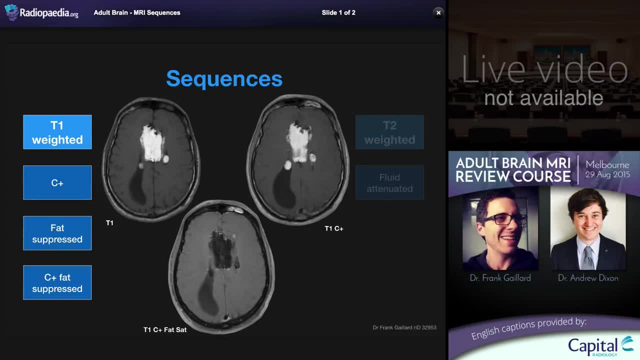 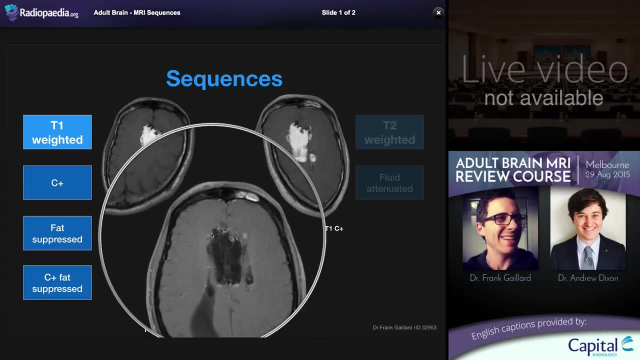 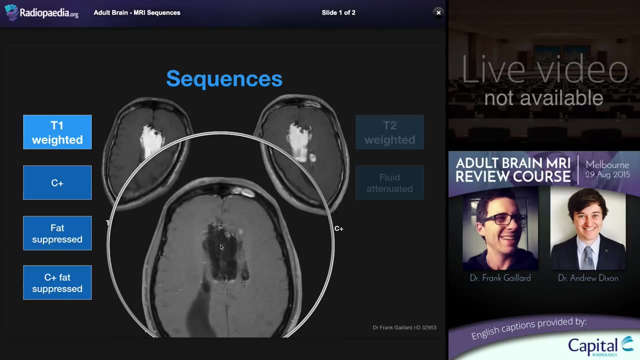 slightly different positioning. So what we can perform is perform fat saturation or fat suppression Where only fat loses signal and contrast remains high signal. And here we can see that at the margins of this tumor there's only very minimal contrast enhancement, with the bulk of the tumor completely attenuating out. Note that in the scalp it's a. 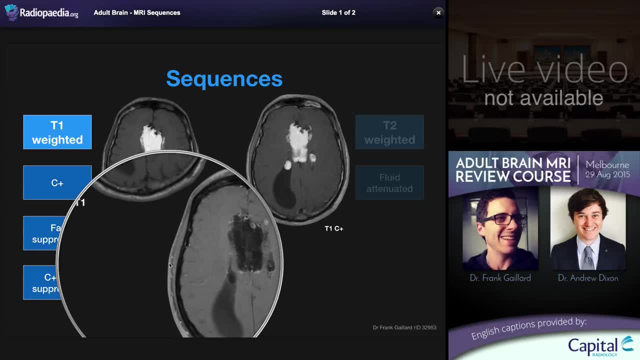 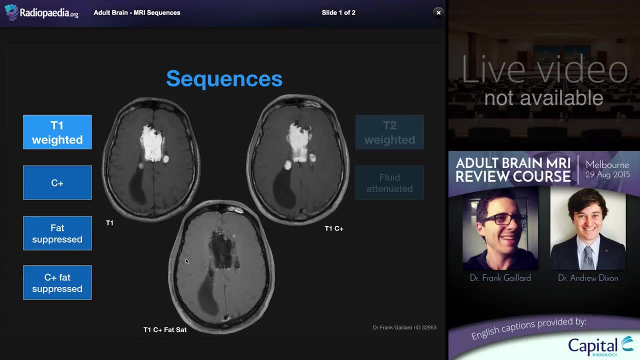 subcutaneous fat that becomes dark, with the scalp remaining hyper intense post contrast due to the administration of gadolinium Fat saturated. post contrast T1 sequences are routine in most parts of the body Because of the presence of significant amounts of fat. this is not the case in 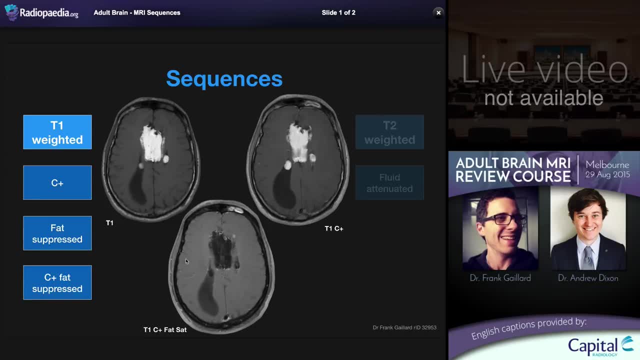 the brain. when fat is an abnormal substance and as such, for purely intraparenchymal lesions, fat saturation is usually not performed. The exception to this is intracranial masses that are involving the skull or skull base, where an extra cranial extension is being sought. So the most common situation for 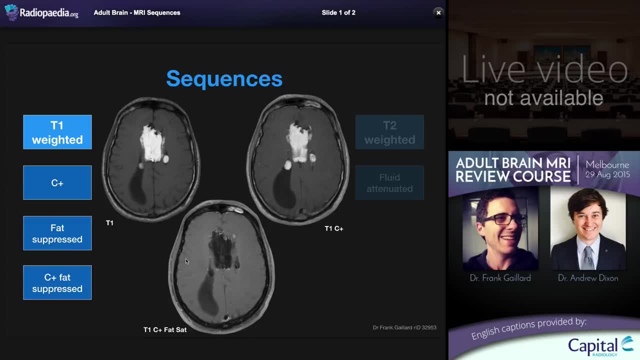 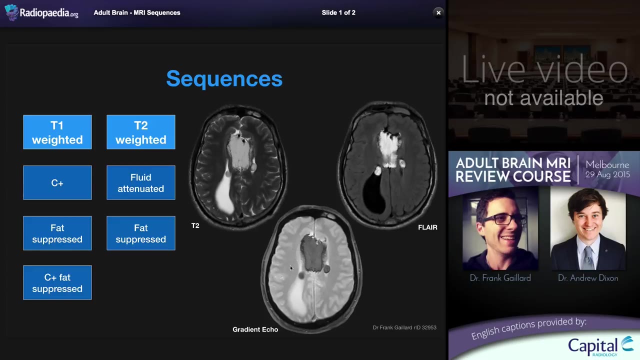 this to be performed would be a base of skull, meningiomas or cerebellopontine angle masses, where potential for extra cranial spread is present. Moving on to T2 weighted sequences, fat suppression is also can be performed. This can be performed as part of a gradient echo sequence where the intention is not. 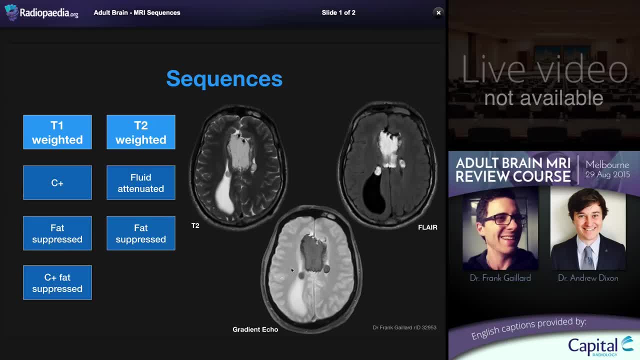 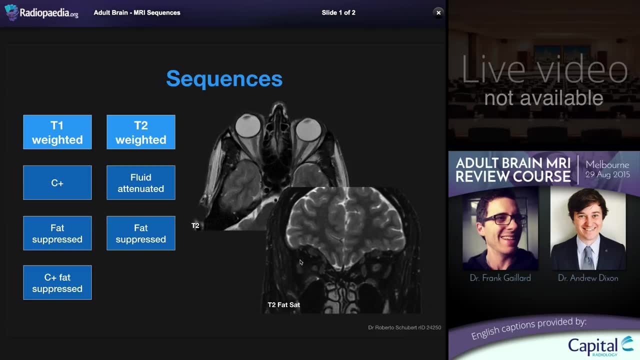 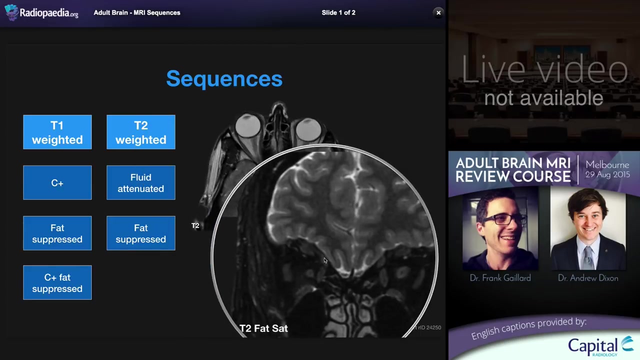 particularly to fat suppress but to make it more susceptible to paramagnetic effects, and we'll talk about that more in a second, Or more commonly, in the orbits or base of skull, to examine structures that are otherwise closely related to fat. This would be commonly the case in the orbits where the extraocular muscles and optic nerve 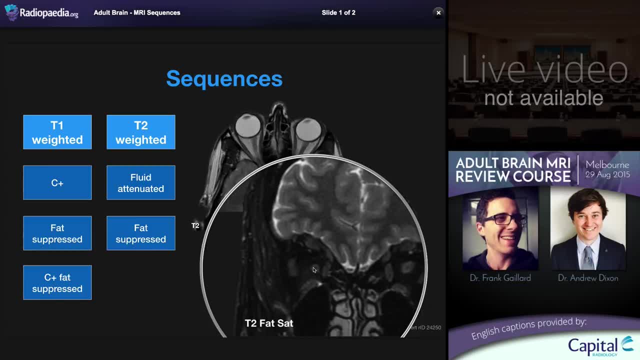 are surrounded by fat, and thus examining for abnormal signal within either of those structures is much more easily performed with the attenuation of fat. The situation in intracranial imaging that this would be useful for would be to look for a CSF leak, for example. 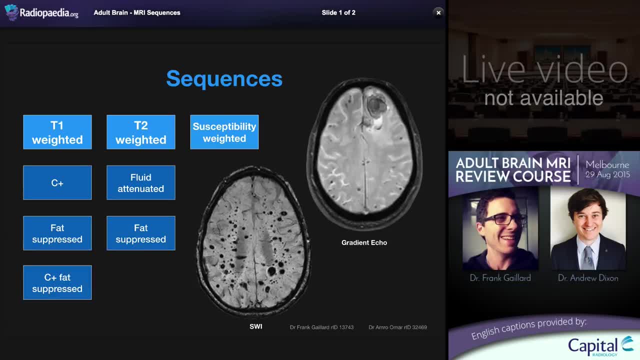 Susceptibility waves. weighted sequences represent a number of different sequences that share the propensity to have signal loss due to paramagnetic or diamagnetic effects. So calcium or blood product will result in dark signal or black signal. The newer sequences, such as SWI susceptibility, weighted imaging, are exquisitely. 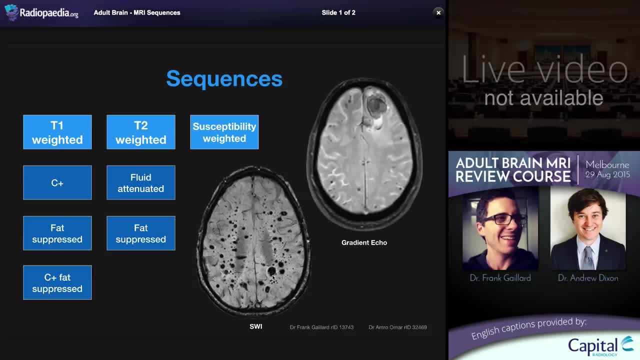 sensitive to very small amounts of such materials. In this example of a patient that has familiar autosomal dominant multiple cavernoma syndrome, we can see numerous large black areas. If you were to look at T1 or T2 weighted sequences, these abnormalities will be much smaller than the ones here, and this phenomenon is 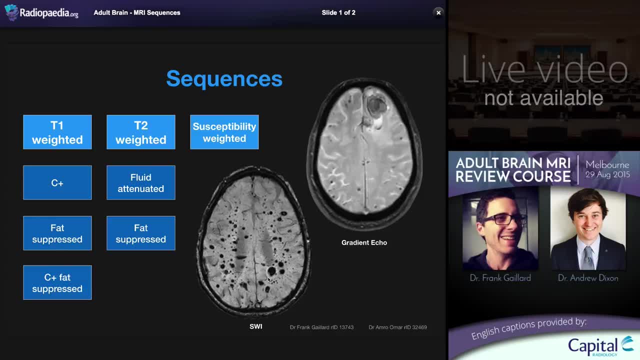 called blooming, where the signal loss extends beyond the anatomical confines of the lesion, and this is due to the fact that paramagnetic or diamagnetic materials distort the magnetic field locally beyond their margins. Susceptibility weighted imaging at higher field strengths is particularly sensitive and earlier and still more sensitive. 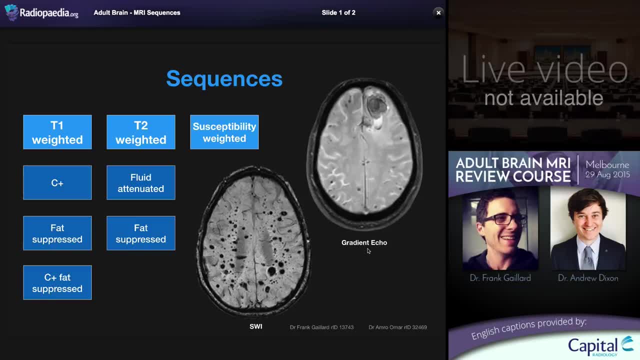 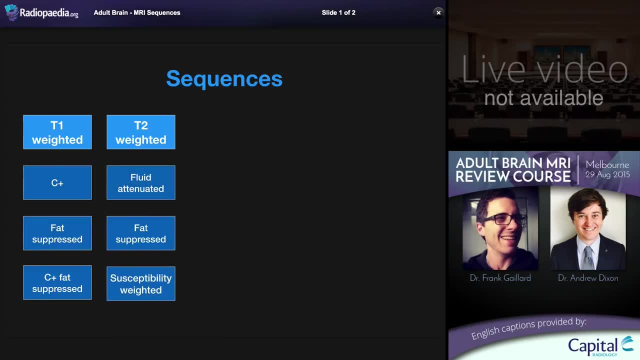 Widely used susceptibility sensitive sequence is gradient echo imaging, but there are a number of others. They probably deserve their own column, but as I'm going to run out of room, we're going to put them under the T2 weighted column, as many of these are T2 star weighted. The next column is diffusion weighted. 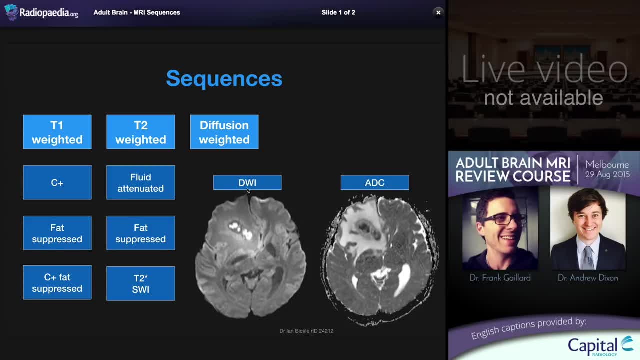 imaging, which really encompasses two main sequences: what we commonly refer to as DWI, or diffusion weighted imaging, or isotropic imaging Or T2 weighted imaging are different synonyms for this- and ADC, or apparent diffusion coefficient. The DWI sequence is really quite a dirty sequence made up of both true diffusion information. 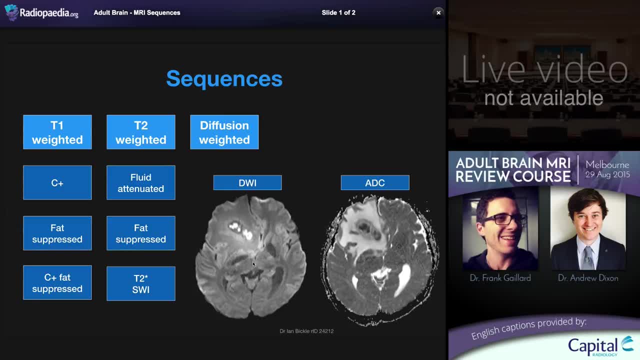 and T2. information and examining the DWI on its own can lead you to erroneously interpret high signal as representing true abnormal, restricted diffusion, when in fact what you're seeing is so-called T2 shine through. The underlying principles as to why T2 shine through exists and the exact relationship between DWI and ADC is well. 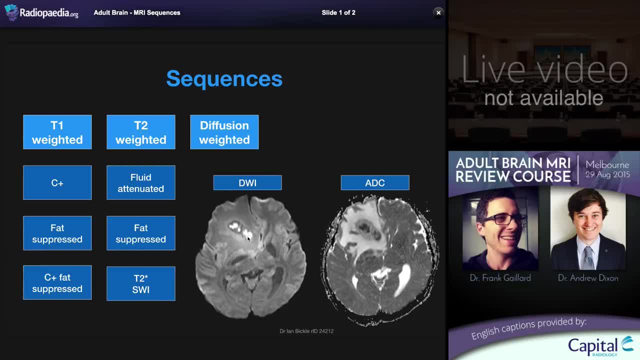 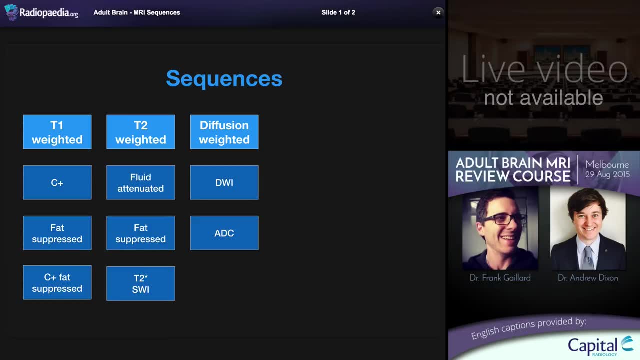 beyond this talk, but I will be creating a separate talk to just examine DWI, because I think it's a very important and often misunderstood sequence. An extension of diffusion is diffusion tensor imaging, which allows tractography, whereby the fact that water molecules motion is restricted along white matter tracks enables the 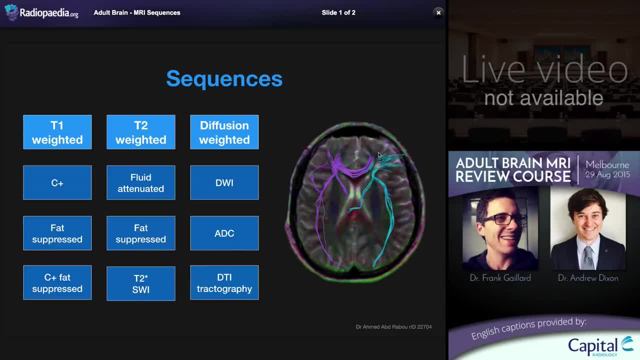 tracking of white matter tracks from one part of the brain to the other, and here we can see white matter tracks crossing from one frontal lobe across the corpus callosum to the other frontal lobe, as well as extending posteriorly, Although tractography is relatively frequently performed, 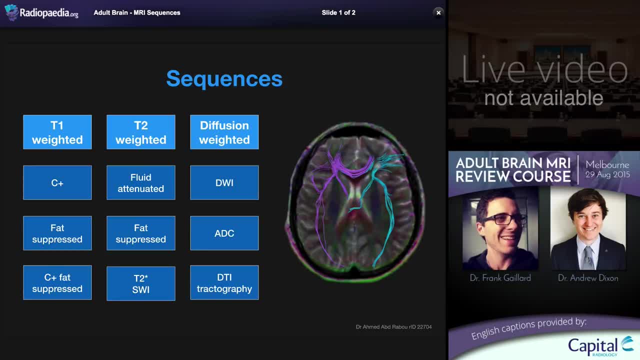 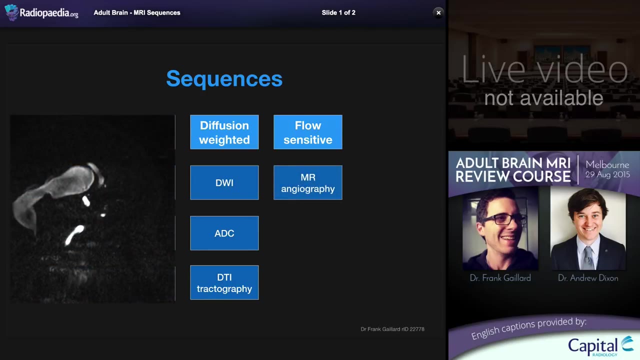 in academic institutions. it's still not really mainstream. Its role is largely research based, but it is finding increasing roles in operative planning. Moving on to our next column of types of sequences, we move into flow sensitive sequences, and these encompass MR angiography, which is usually 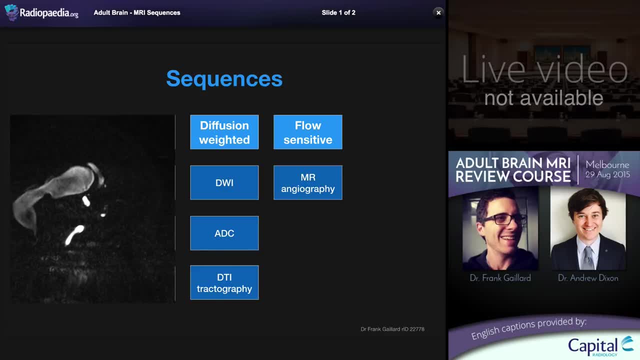 performed without intravenous contrast and relies on blood bringing with it signal. These can be shown just as a stack of very thin images, and because there is little background for the vessels to be localized against, it can be difficult to know exactly where one is on a single image. Thus, often these images are shown as a stack of very thin images. These are often shown as a stack of very thin images and because there is little background for the vessels to be localized against, it can be difficult to know exactly where one is on a single image. Thus often these images are shown as: 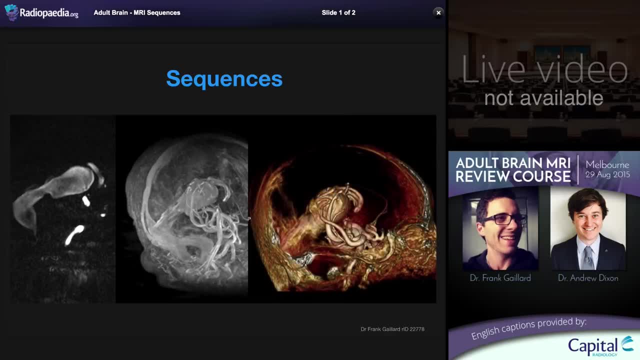 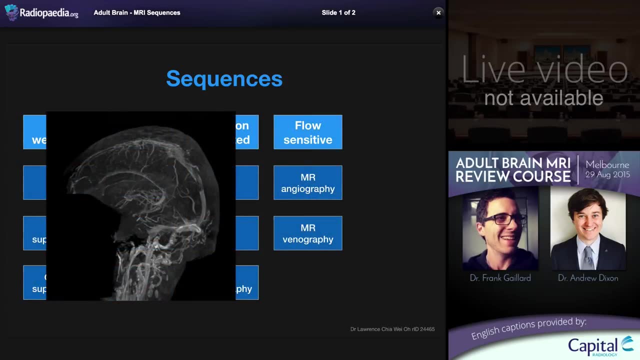 MIPS- in this case of a young patient with a vein of Galen malformation- and these can of course, be surface shaded. MR venography can be performed similarly to MR angiography or also by other techniques such as phase contrast, and can be used to image dural venous sinuses and cerebral veins. 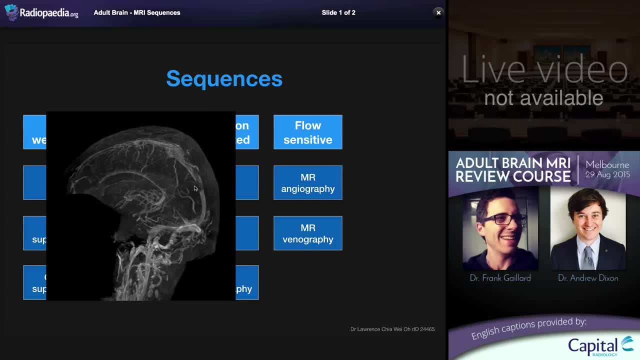 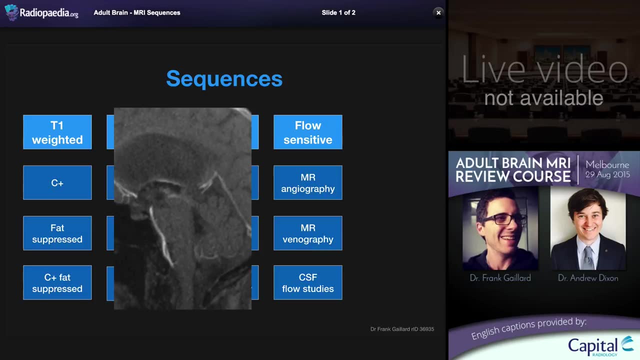 Here we can see thrombosis or occlusion of the posterior part of the superior sagittal sinus, and the same principles as phase contrast venography can be employed to look at the pulsatile flow of CSF in the cisterns and the aqueduct, as shown here. 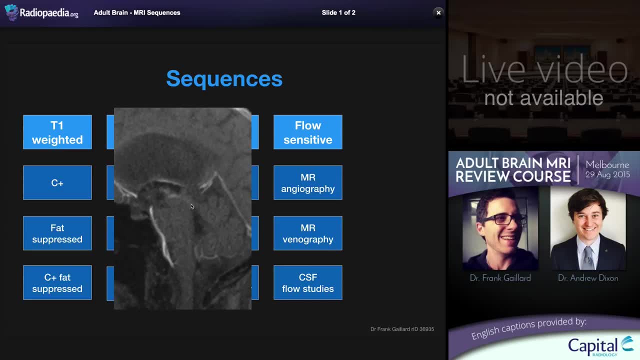 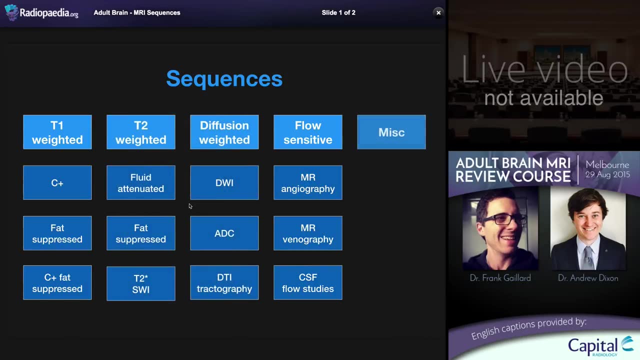 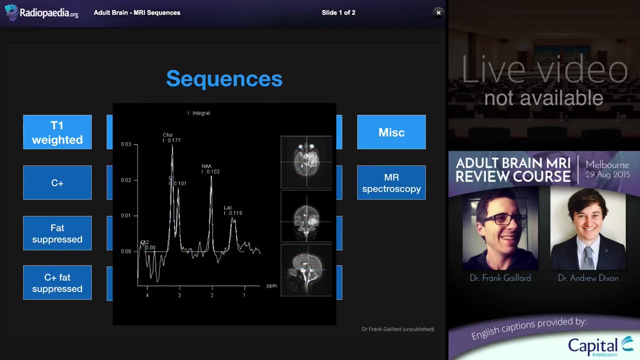 This can be particularly useful if aqueduct stenosis needs to be excluded or if hyperdynamic flow of normal pressure hydrocephalus needs to be evaluated. And on to the last column of miscellaneous sequences, which includes MR spectroscopy performed very routinely as part of a particularly brain tumour or mass work-up.